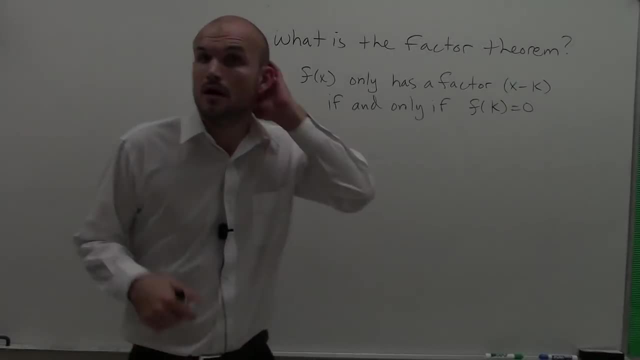 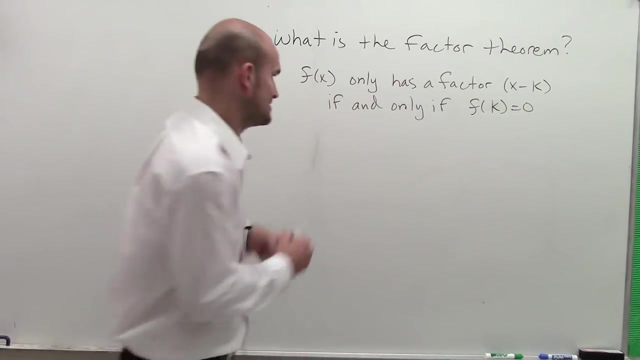 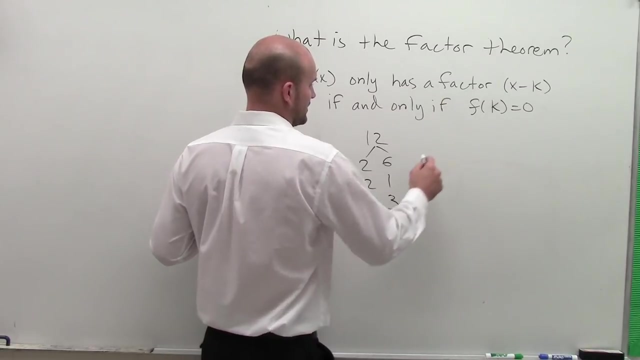 All right. so if you watch my video on remainder theorem, the remainder theorem helps us understand the factor theorem. Now remember factors. Let's take a look at all our factors of 12.. Factors of 12 are 2,, 6,, 12,, 1,, 4,, 3, negative 2, negative 6, negative 12, negative 1, and. 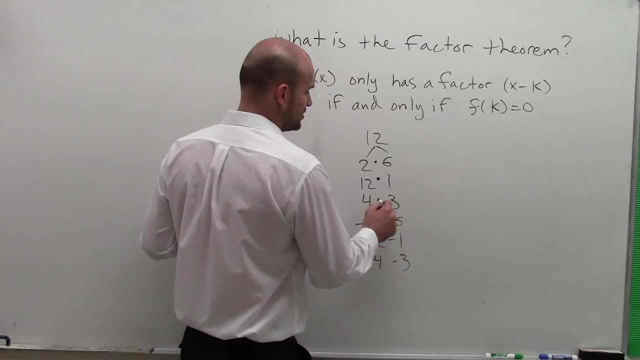 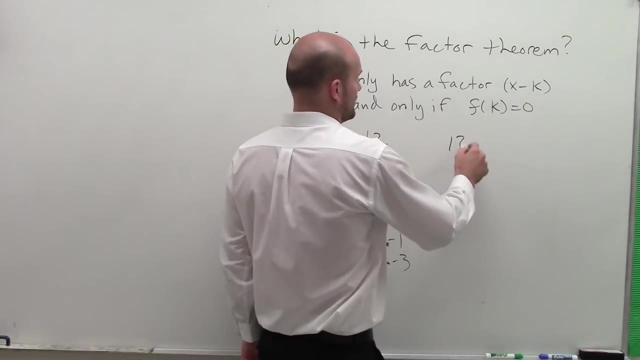 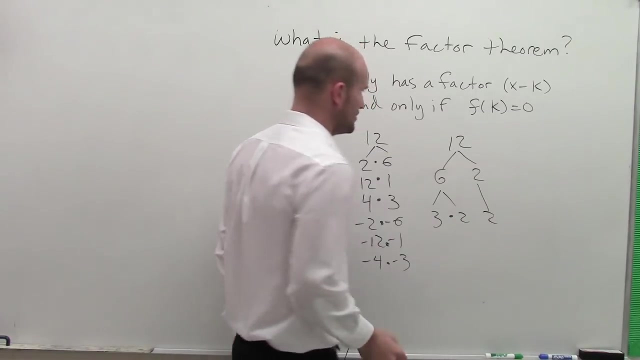 negative 4, negative 3.. And they're factors because they multiply by each other, right to give us 12.. We could also look at, remember we talked about, like the factor tree, You know, you could break it down into 6 times 2,, 3 times 2 times 2, and you could also do. 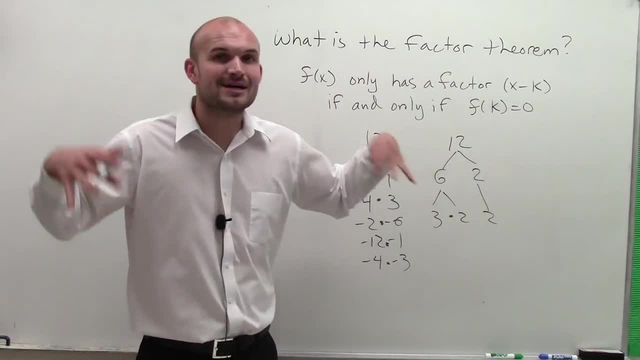 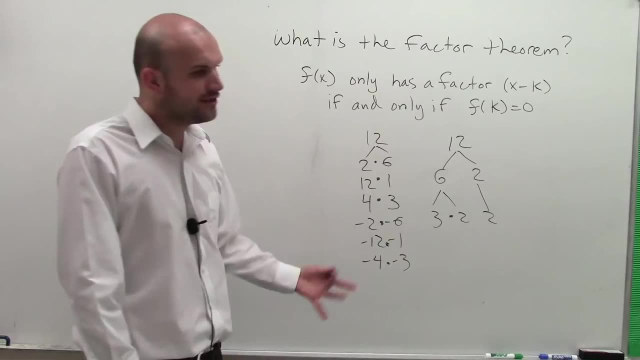 4 times 3, and then break it down to 2 times 2.. But we're breaking them down into our factors, numbers that multiply to give us our resulting number 12.. Now the other thing to think about: a factor: all of our factors evenly divide into our number, right? If it's not, then 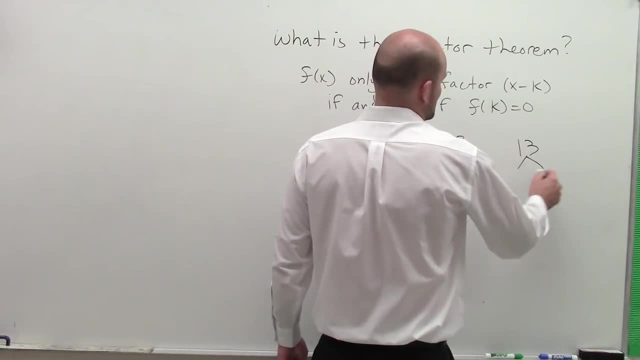 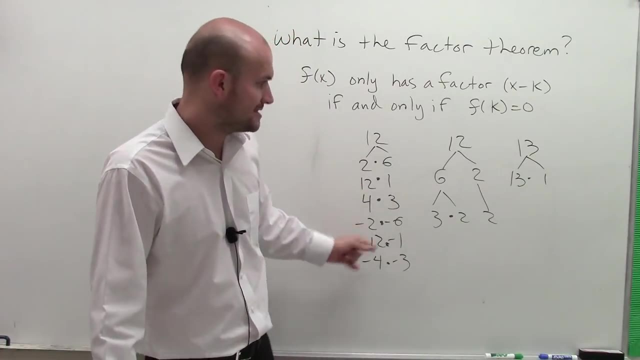 they're not a factor. Let's take the number like 13.. The only factors for 13 are 13 and 1, because those are the only two numbers that evenly divide into 13.. You can't take any of these numbers and divide into 13, because you're. 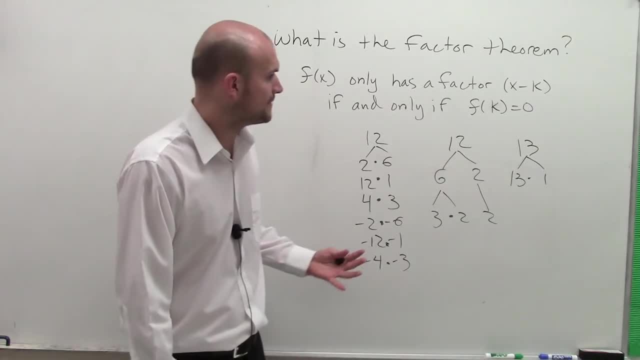 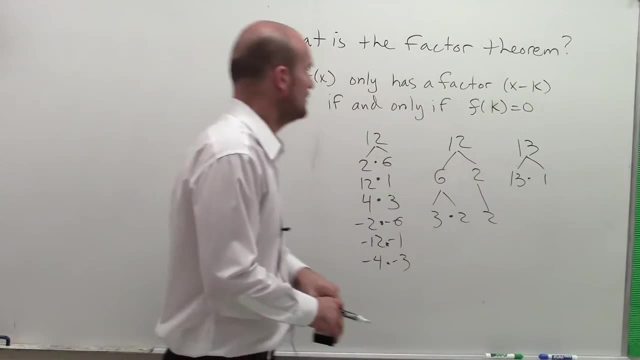 going to have a remainder right when you think about dividing into using division. So all factors, all the factors of a number, evenly divide into a number. Well, that's going to be the same thing. So when you evenly divide, that means you have a remainder of. 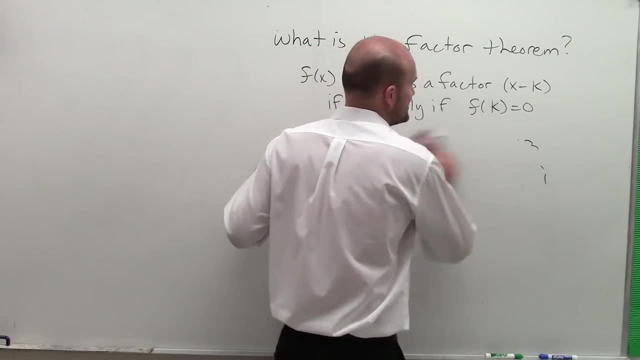 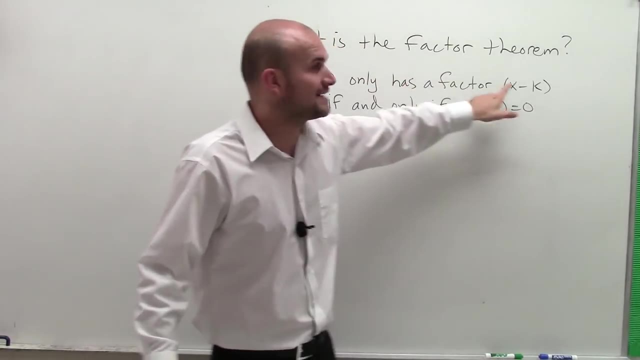 zero right? Well, by the remainder theorem. if our remainder is zero, then we know that we have a factor. Well, think about it. If, by polynomial f of x, for it to have a factor x minus k, then I have to apply the remainder theorem. That means x minus k has to evenly. 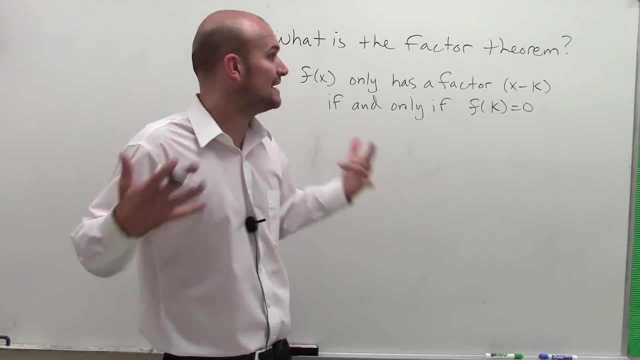 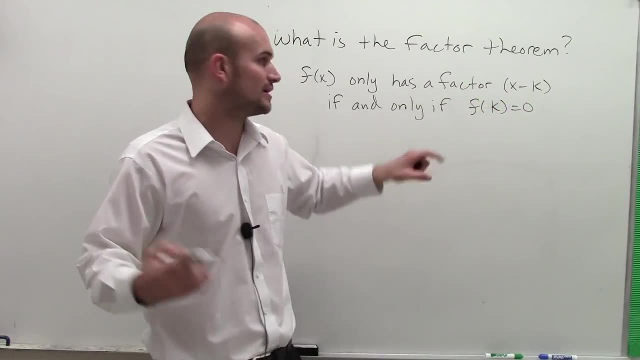 divide into it. So the only way I know that it is a factor is well, one, by using synthetic or long division and you get the remainder of zero, or by using our remainder theorem when we plug in the zero into our function and we evaluate our function for that zero. when we get zero, we know that we have a factor. So if we plug in the zero into our function, we know that we have a factor. Well, think about it. If, by polynomial f of x for it to have a factor,